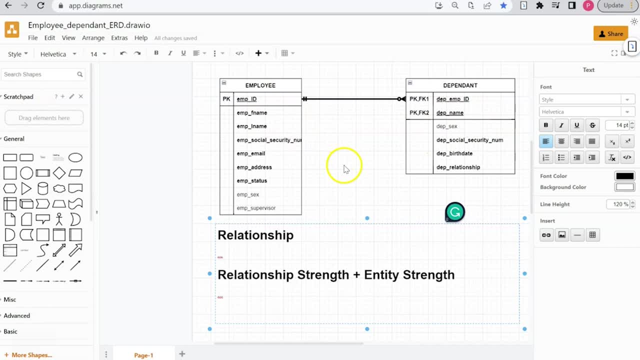 And dependent. so I want to step back. We'll talk about the keys in just a second, but let's step back and actually write the relationship between an employee and independent, Talk a little about the strength and then discuss the type of keys we see within this diagram. 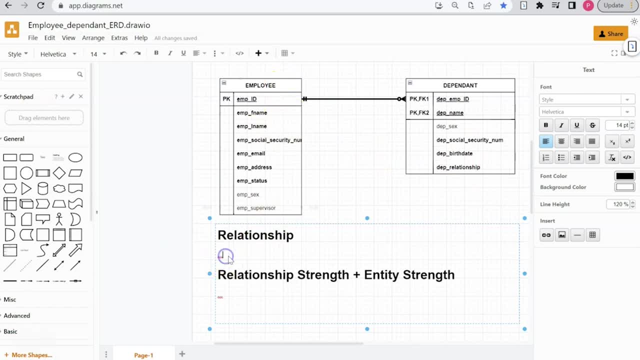 All right, so let's go ahead and write the relationship. So I'm going to step down here. say is that an employee can add the add is our verb, add zero or more dependents, And then here we'll say the bi-direction will be: each dependent can add, can be added by. 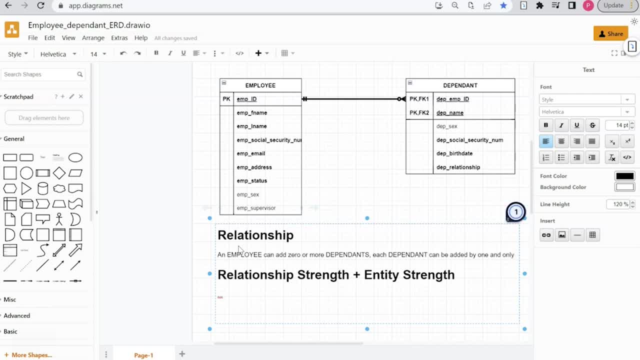 one and only one employee, right. So that's our relationship that we have here. We have the cardinality, which is an employee can add zero or more, And then the bi-direction is that a dependent can be added by one and only one employee. 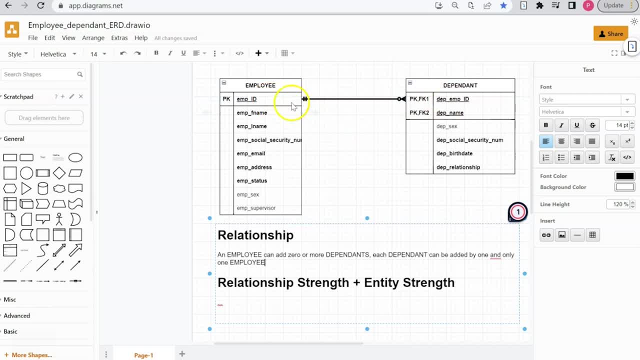 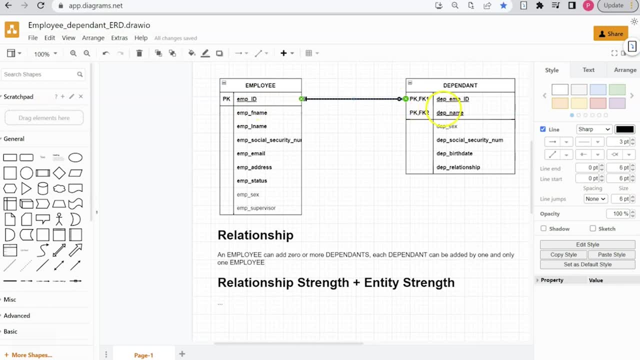 Now, the relationship here between an employee and dependent is strong, And so that's indicated by the solid line between employee and dependent. And the reason why the relationship is strong is because if we were to delete employee, we're going to delete All of the corresponding dependents. 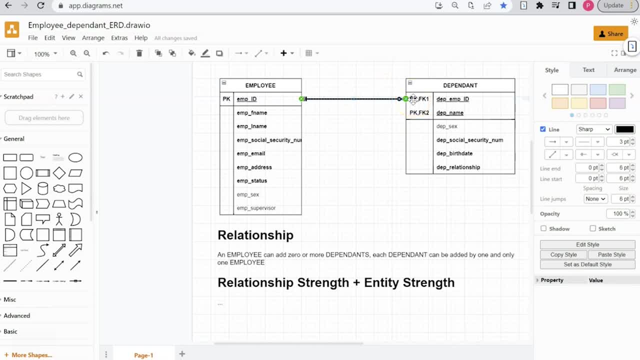 So you don't want to leave. as I say, for instance, you have an employee and the employee has a spouse and two kids. If that employee leaves the company, we also want to delete that employee spouse, as well as the two kids, from the database as well. 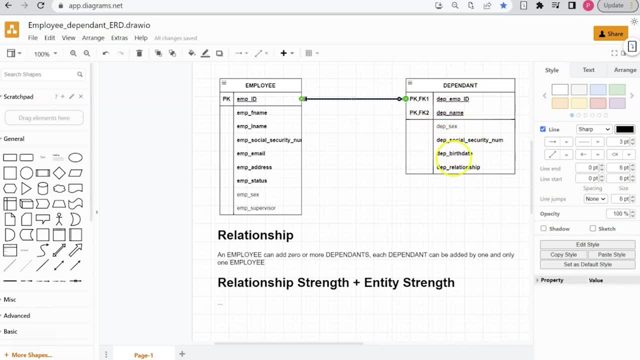 Um, so dependent is what we consider a weak entity? Uh, it's existence dependent upon the employee. So if we get rid of an employee record, we want to get rid of all the corresponding uh dependent records that are associated with the employee. 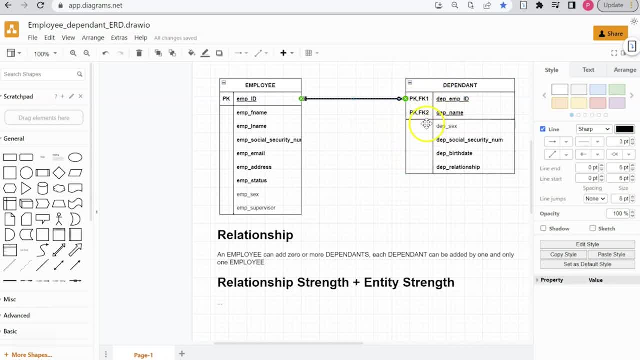 And that brings us to the key. We have a composite key that makes up and which uniquely identifies each row, And so we have the employee ID and the uh, the dependence name, which is a composite primary key uh that would uniquely identify the dependent. 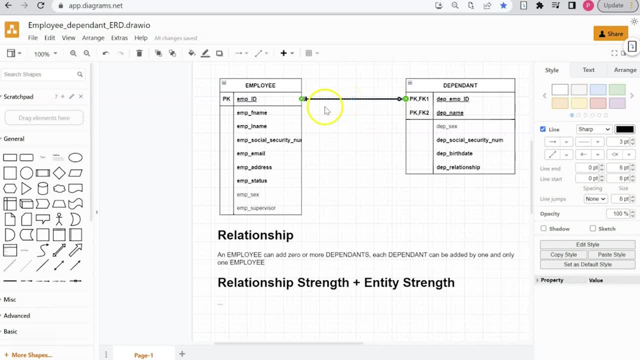 Um, and, like I said, with relationship strength- and we notate that with a silent line, whenever we delete an employee, we want to, uh, retroactively go back through our database and delete all of the folks who are associated with that employee. 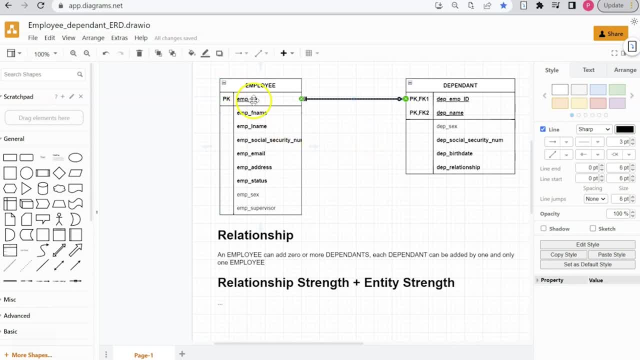 So, um again, just to reemphasize, uh, employee is a strong entity, Dependent is a weak entity and we can usually identify that, sometimes through the composite key, but the relationship is strong. Uh, in a sense that if we we notate that with a data, I mean with a solid line, and 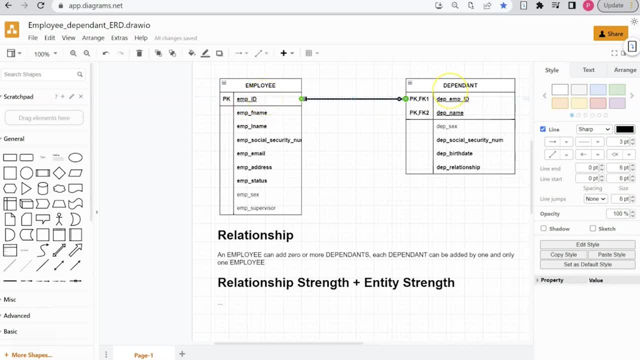 if we were to delete an employee, we would delete all the corresponding dependents. Now, the last thing I want to focus on here is that primary key uniquely identifies a row uh for the employees. We can have hundreds of employees, but we can identify the first name, last name, social. 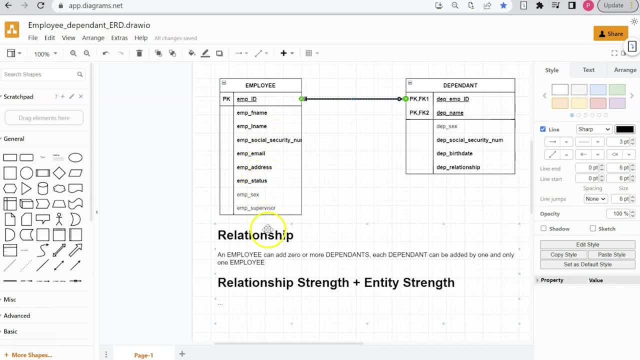 security number, email address, status, sex supervisor- All by the employee ID. We can do a search and look up a unique instance of an employee by the employee ID number. Now we also have an alternative primary key or our alternative key. 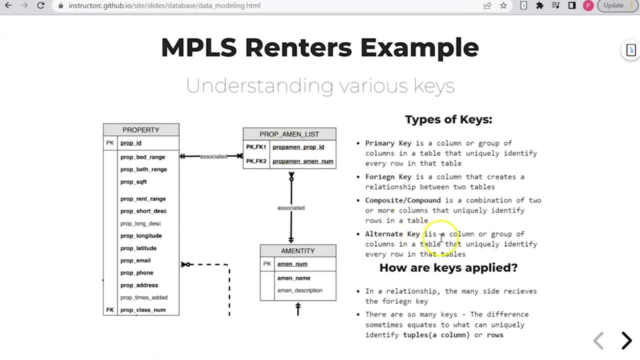 And so, if we look back at our slides here and our turn of key, you need to correct this here. It says is, but it should be: is a column or group of columns in a table that uniquely identify every row. So this alternative key does not serve as the primary key. 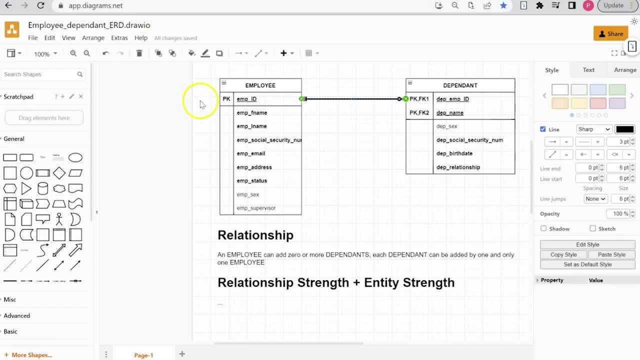 But if we needed it to, we could. so we could swap out employee ID for employee social security number, because it's a unique number that will uniquely identify the employee. But most companies are moving away from using a social security number to uniquely identify.